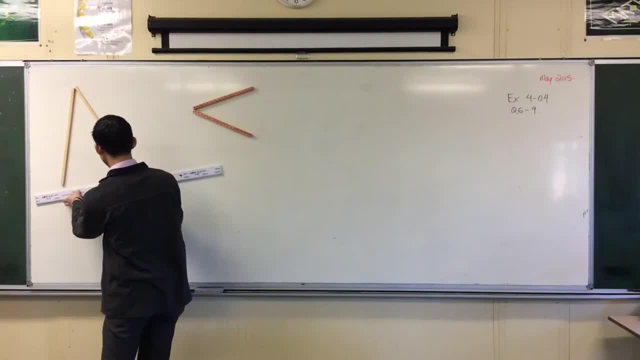 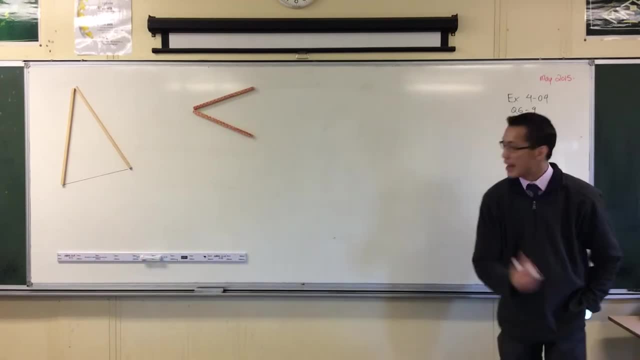 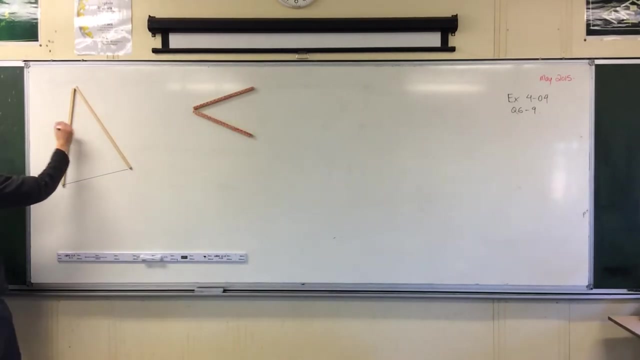 So let's just do it for this one. Here's an example. Okay, so I have my triangle now. Now, hopefully, as you went through it, as you measured, you would have had some lengths up here. I think I had something like this: five, five, and then this would have been three. 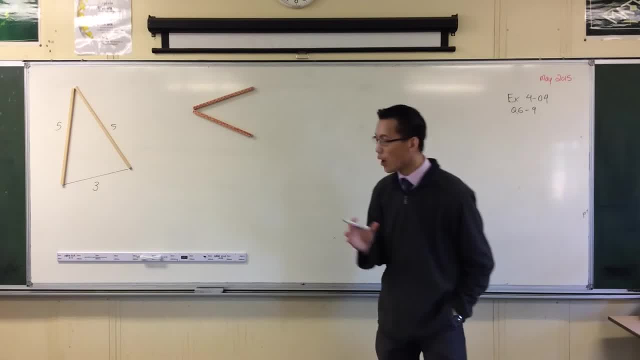 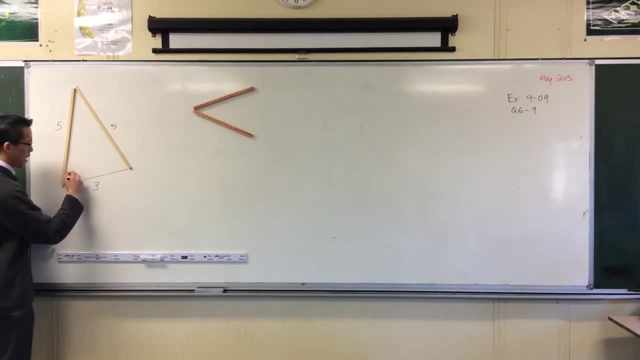 And then you went and you did some angles. So here's what I measured: while you were all working, I measured the one that I had on the ground, on the table, And this is what I got. I have my 71 degrees, 35 degrees and 71. That's what I measured. 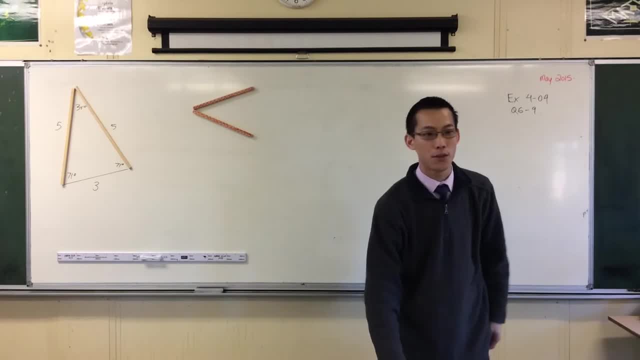 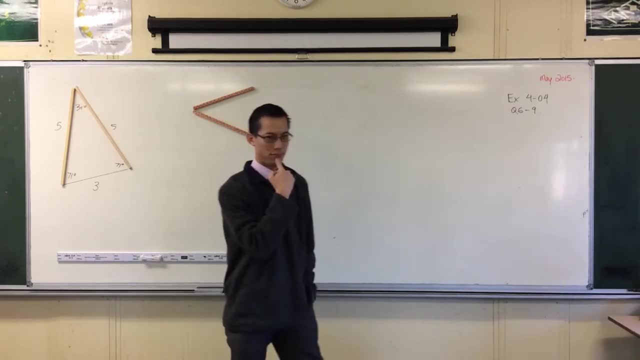 Now, before we make any conclusions through this, let's just look at it and notice a few things. Number one: if you add up these angles, if you add up these angles, look at them with me now. What do you get? What do you get? Yeah, Brandon. 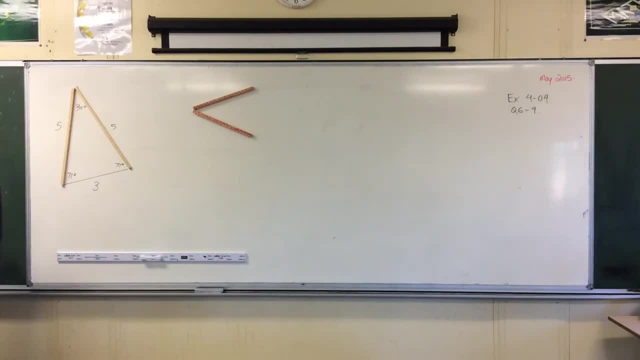 Okay, now you're expecting to get 180,, aren't you? We have learnt that the angle sum of a triangle Is 180 degrees, but if you have a look at my numbers, let's just do one at a time. 71 plus 35 is 106, because there's one thing: 106 plus 71 is 177, with three degrees off. question mark. 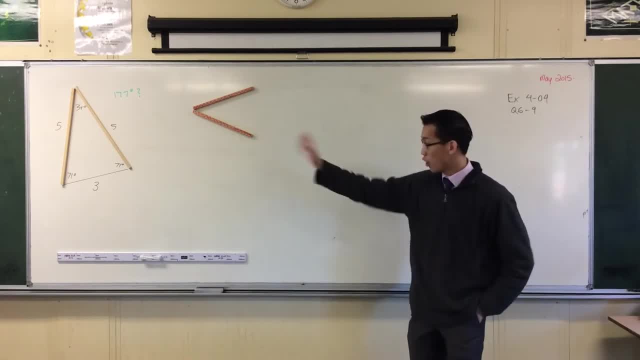 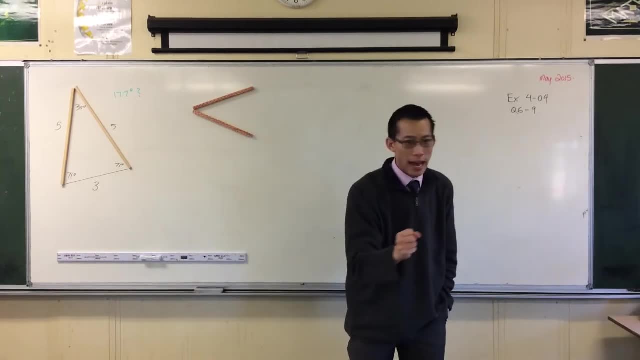 Okay, now legit question. This is not the main point I'm making, but I hope you arrived at something similar. You add it up and you're like: I don't have one, It's 180.. Okay, now question, and I can think of at least two answers to this. 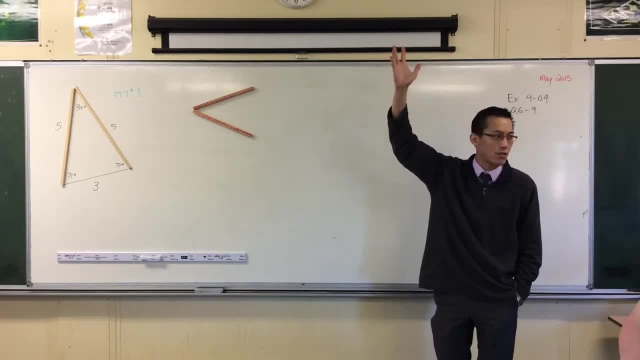 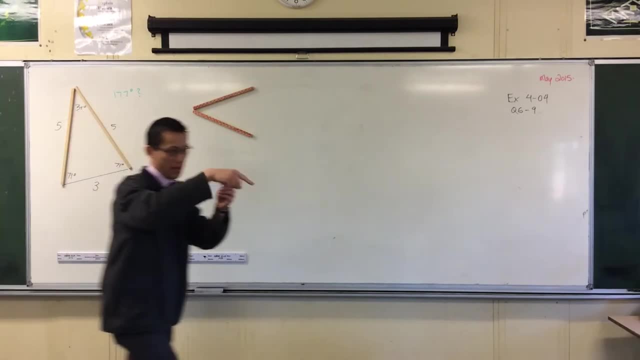 Anyone want to raise their hand and suggest: why don't I have 180 degrees? Okay, first attempt. yeah, Um, an accurate measurement? Okay, excellent. So I'm going to pitch one of these. So put your hand down for a second. I'll come back to you in a second. 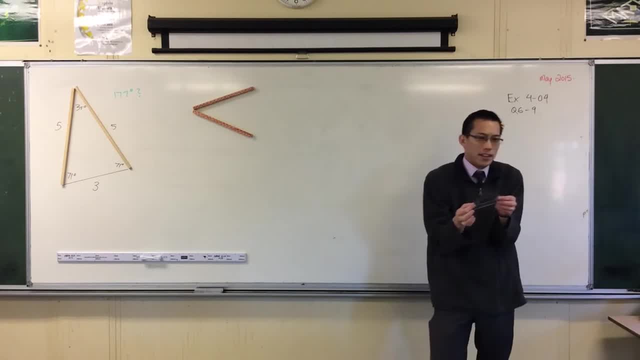 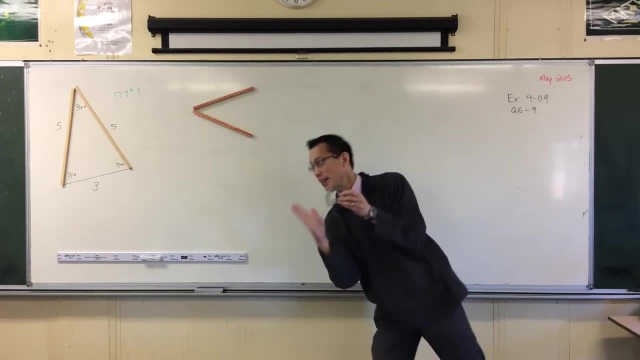 You've got this instrument here right And well. it's not perfect And you can only measure so well like my, eyesight is terrible. So you know, between one degree, I'm not sure if it's 20,, 35.1 or 35.2.. 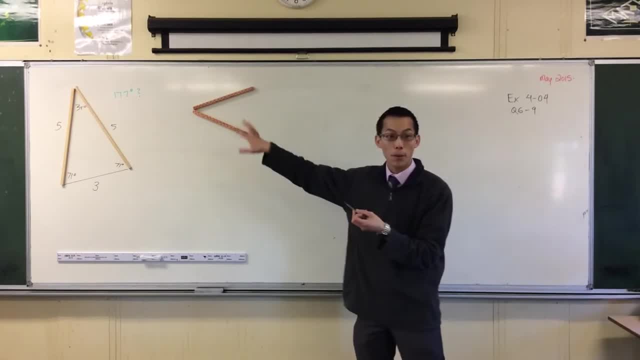 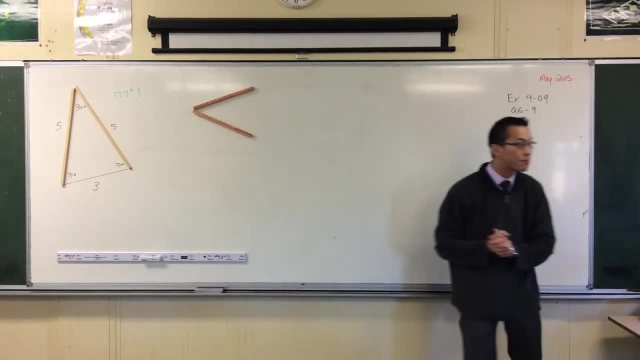 Can't tell, So I'm only so accurate. We have what we call here limits of accuracy. Okay, there's the first suggestion, So I want to give me another one. Yeah, yeah, yeah, yeah. Um, is it because you're using, like the squares? 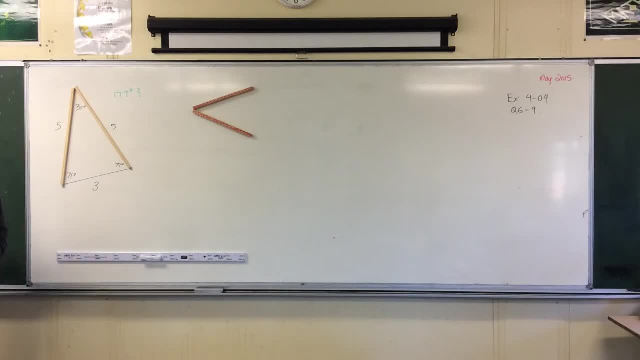 And like because they're all like, you can't get it really perfect, Like as you can see on that one now there's a gap. Perfect, Yeah, absolutely, And it's hard to keep it still. Exactly right. 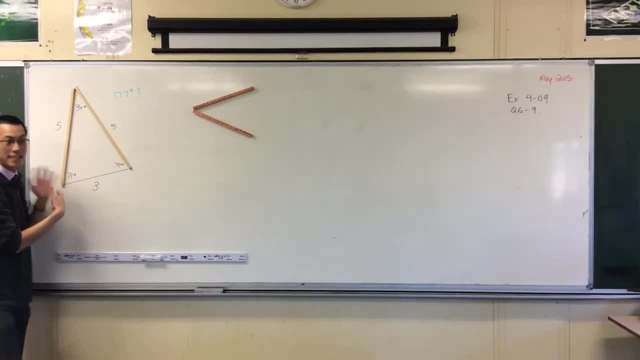 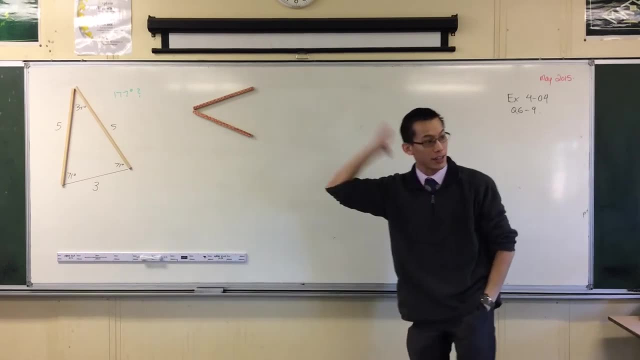 So, number one, the instrument I'm using has a limit. But number two, like we've constructed something And it's not perfect. Do you remember we were talking about Euclid a few lessons ago? right, And his introduction to geometry? 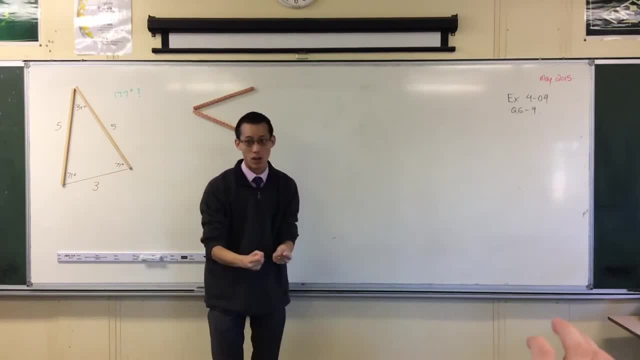 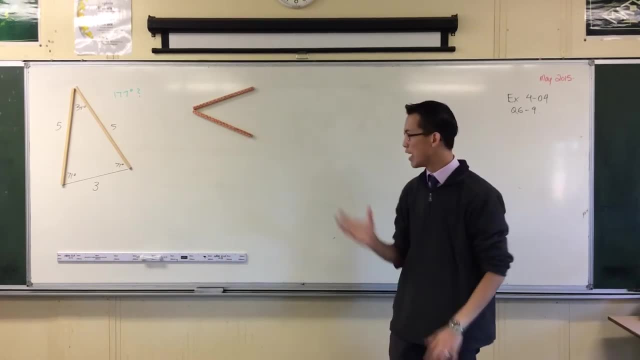 He knew that this wasn't perfect, But he imagined a world where it was, And in that world every triangle adds up to exactly 180 degrees. You can measure everything perfectly. It's not the world we live in. That doesn't mean it's not real. 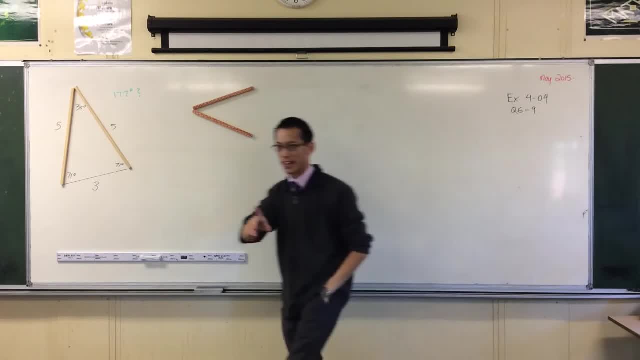 Okay, All right, now let's move on. Here's what I'm interested in looking at. Okay, yeah, There is also another one where we found that when you're trying to measure them, they move around. Yes, Yeah, that's what I said. 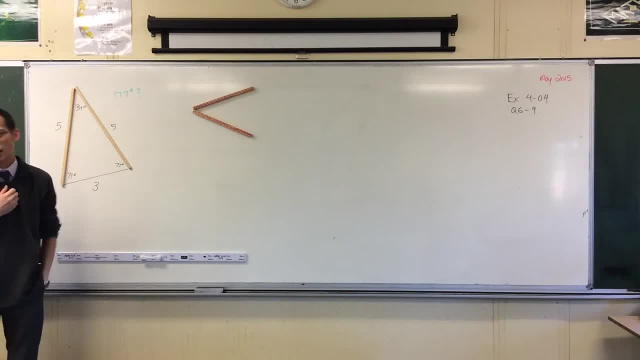 Yep, yep, good, good Again. I put that under limits of accuracy, I think, because we're just human beings, Yeah, Okay. So now here's the thing that's interesting. okay, Have a look at your angles. 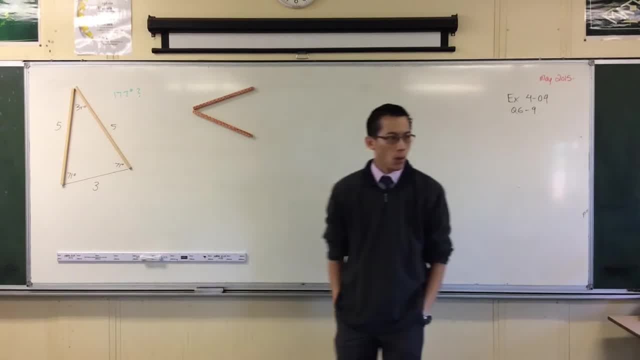 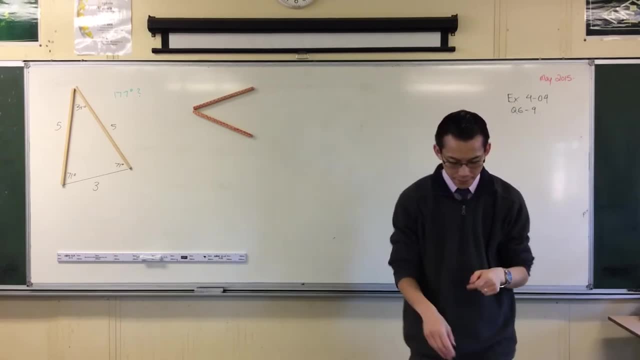 What do you notice about them? What do you notice about them? We started with two equal sides, right. That was how we constructed this shape. What did we end up with? Yes, We always ended up with like a triangle that kept getting larger and larger. 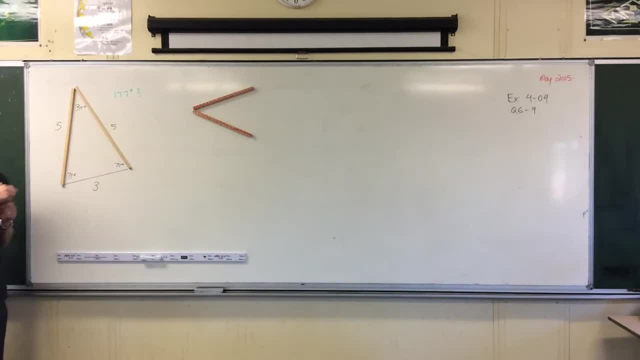 Okay, all right. So you might have been changing up. ladies and gentlemen, I'm going to change this in a second. What I can see in addition to that is that these angles here, in these corners, right, they're always equal, right. 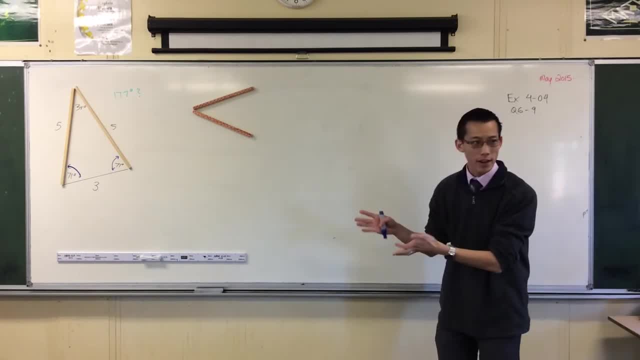 We started with equal sides and what you end up with without a choice is you end up with equal angles. If they're not equal, that's down to just limits of accuracy. when you're measuring right, Not only are they equal, but can you see, they're always down here. 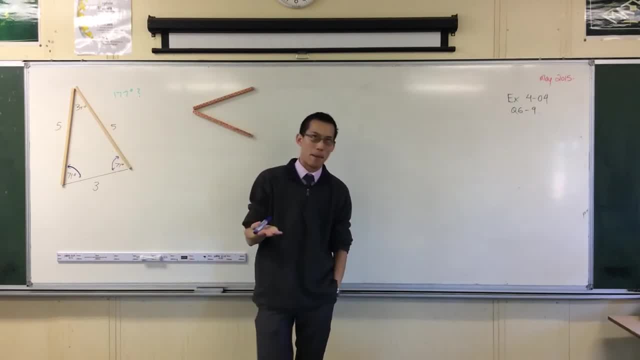 It's never this one up here, except by coincidence. If you, you know, by coincidence, For instance, make an equilateral triangle, because then they're all equal, It's always these guys, It's always the angles. Mark this. 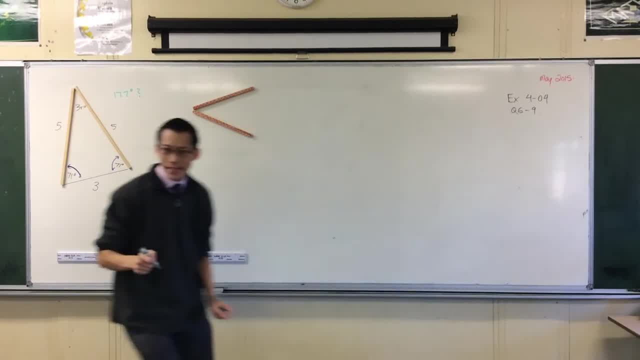 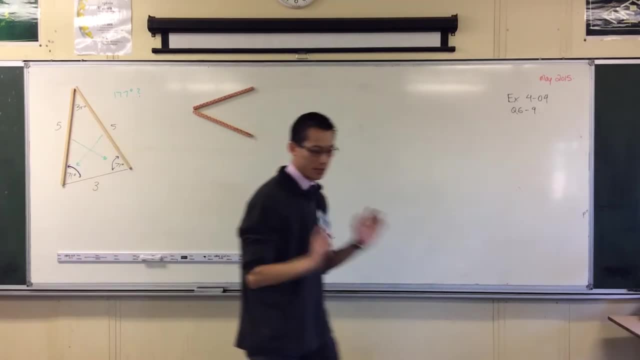 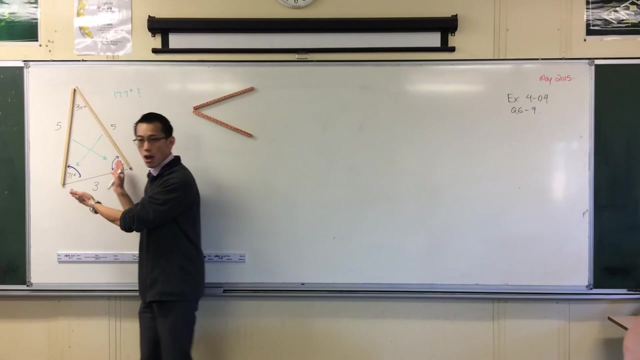 This is really, really important: It's always the angles that are opposite the equal sides. That's so important. I want to say it again and, in fact, I'm going to ask you to write it down, okay: Every time you have a triangle with equal sides in it, you get equal angles, and the equal angles are opposite equal sides. 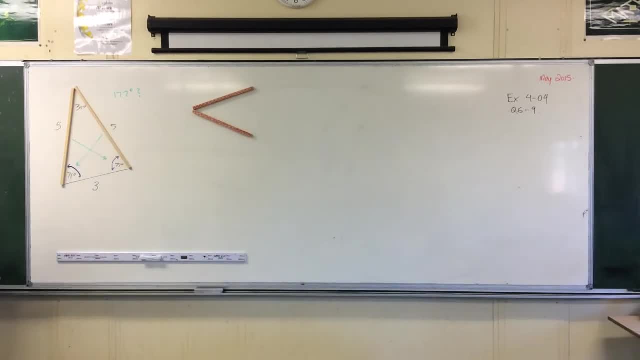 I'll write that down. I'm going to write that down as well, and so should you. Yes, How do you know that they're opposite? Because how? oh, because it's Okay. so I'm looking at their position, okay. 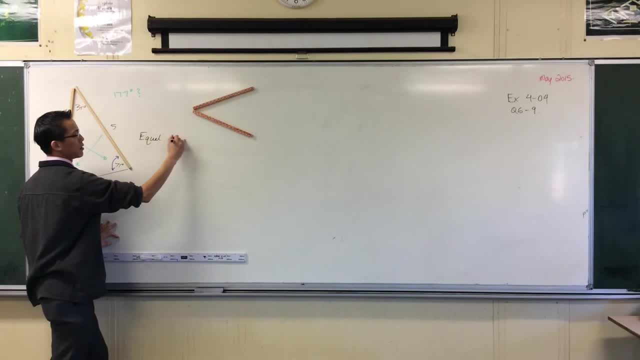 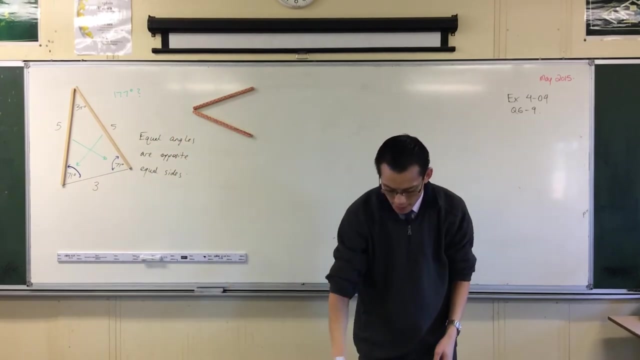 So let me write that down: Equal angles. equal angles are opposite equal sides, and you have to be right. Let's have a look at this triangle over here. okay, It's a bit smaller, but I can do the same thing, right. 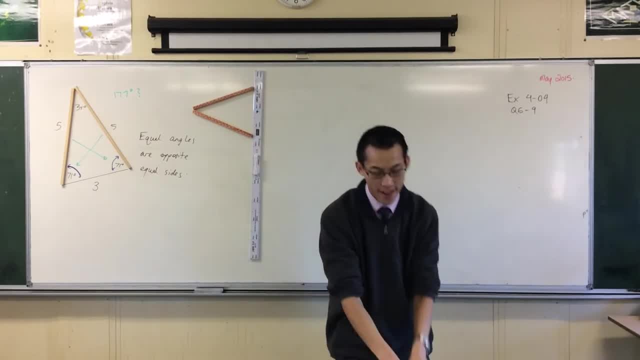 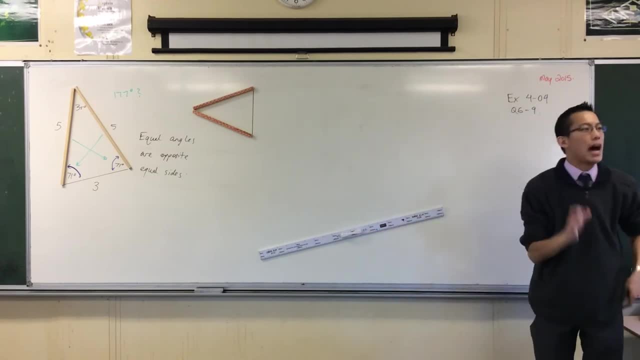 Will I put this up, Are we? Yeah, okay, And I mark out my third side, the one that's not equal to the other two. right, Even without measuring, you can see there's a smaller angle over here, right? 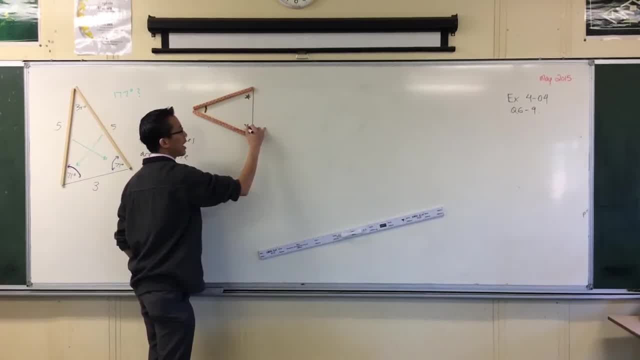 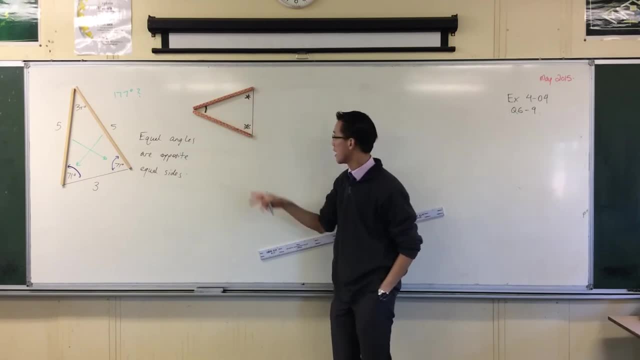 And then there's these two guys who clearly are the same size, and measurement will confirm that. okay, It's not only when there's one small one and two bigger ones. right, Let's just I'll complete this triangle, put it over there. 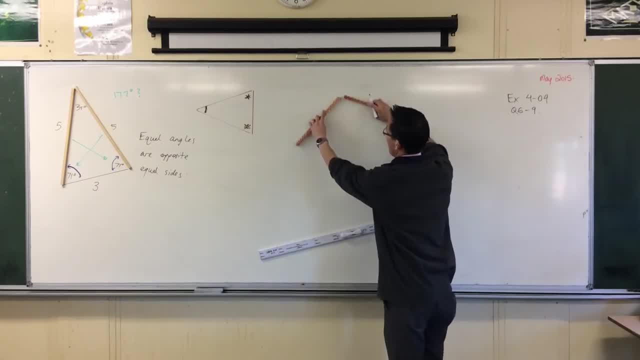 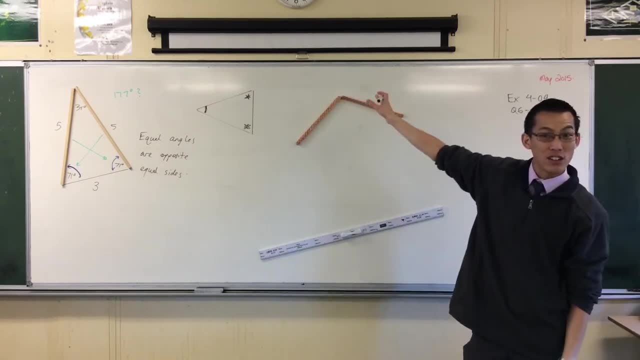 If I now take the same sides right And I make the angle between them really, really large. So think of angles now. What kind of triangle is this? with regard to angles, It's an obtuse triangle. very good, because that angle's huge right. 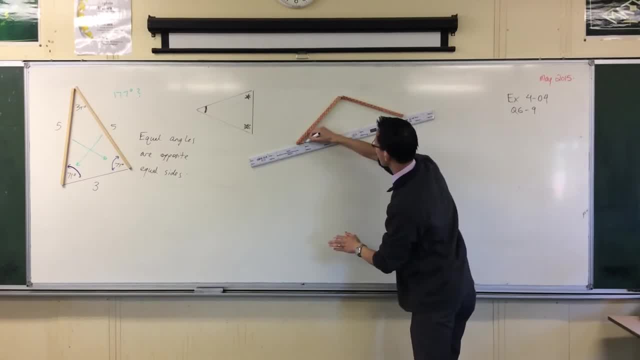 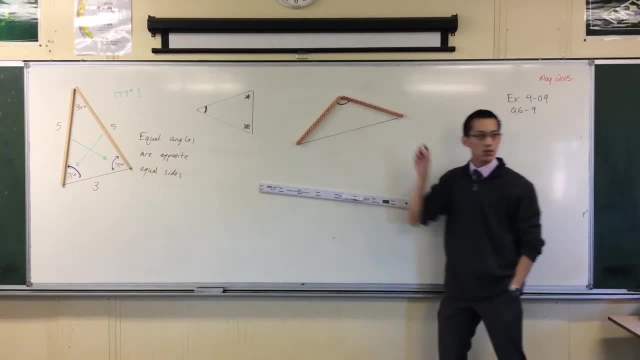 Now when I make this third side, there we go. That angle up there is obtuse. like we said, it's huge. right, You have these two smaller angles, but again, you can go ahead and measure and you actually did. 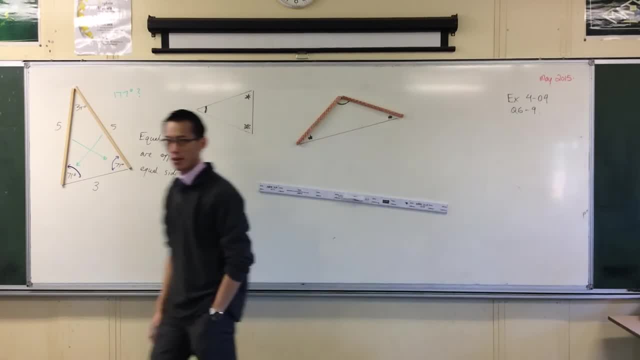 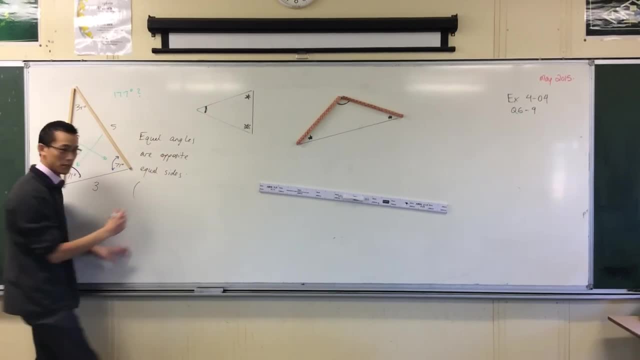 You will find that they are equal to each other. okay, Equal angles are opposite equal sides. You will see this written another way as well, So you can put this underneath this. right, We've been making isosceles triangles, right.